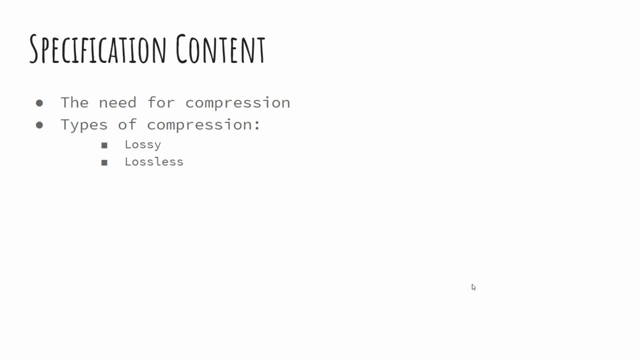 the need for compression and the two types of compression. So we have lossless and lossy as types of compression. You need to be familiar with those two types of compression and actually when they're most appropriate and what the uses are. So we'll cover those off in the course of. 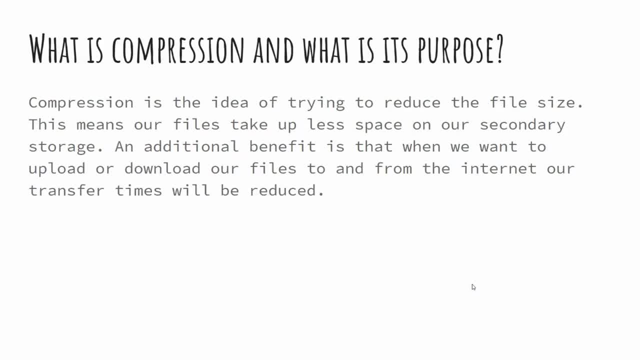 this presentation. So, firstly, compression is the idea of reducing a file size. So it could be, for example, a photograph. Reducing the quality of that photograph will reduce the file size. So, for example, if you think back to our lessons where we looked at how images are represented, 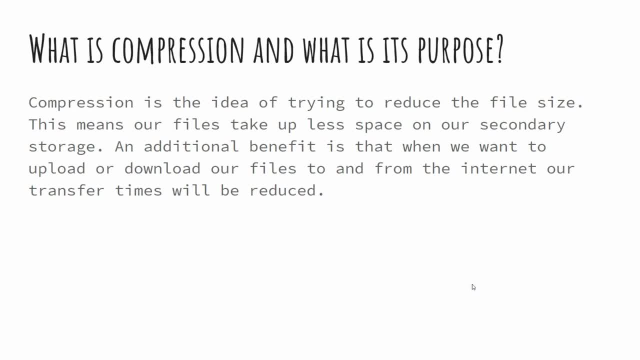 using binary. if you remember that we were saying about that, there are bits behind each pixel that define how many potential colors there are. We could reduce the number of colors, therefore reducing the size that that image takes up, but that is at the cost of quality, And it's about that trade-off between the cost of quality versus 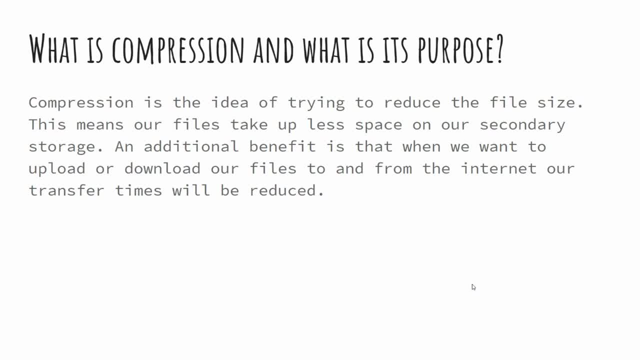 file size. But compression is all about removing data to make it take up less space on our computer. Now, the additional benefit of reducing the file size is also that it makes it far, far quicker for us to be able to transfer that data across the internet. So in a world where 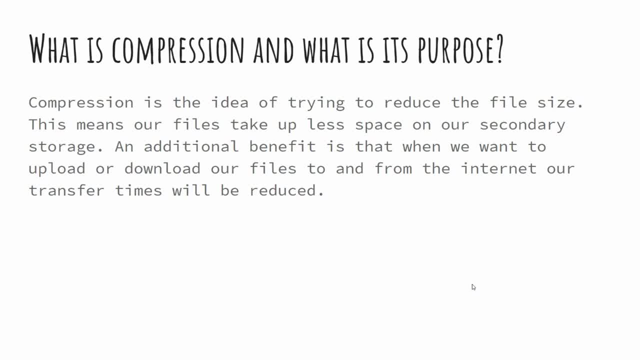 we're living much more online now. if our file sizes are reduced, it means that we can download them and upload them and send them across our networks much, much quicker, reduces the amount of bandwidth that we're using and generally just speeds up the whole process. 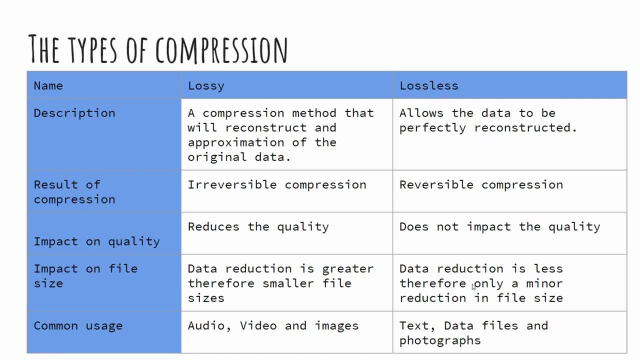 As I mentioned, there are two main types of compression. We have lossy and lossless. Now, lossy compression is a method of compression that you will remove data, as I mentioned, for example, color from images or resolution from a video file, as an example, and that 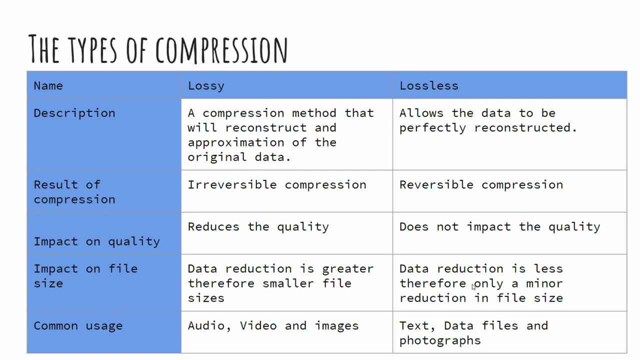 information will then in essence be deleted and lost, So it won't be data that you can restore. So it's an irreversible type of compression. It does reduce the quality of that file, But generally speaking, when we think about things like files like audio, video or images, you can afford to reduce the quality and still have the 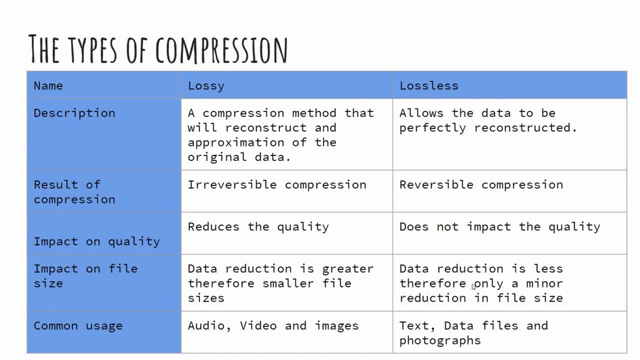 information that you're trying to present being able to be understood. If you think about videos on YouTube as a really good example of this- watching a video in 1080p, so full HD, versus watching it in 720p or just standing in front of a computer- it's a really good example of this. So it's a really good example of this: Watching a video in 1080p, so full HD, versus watching it in 720p or just standing in front of a computer. it's a really good example of this: Watching a video in 1080p, so full HD. 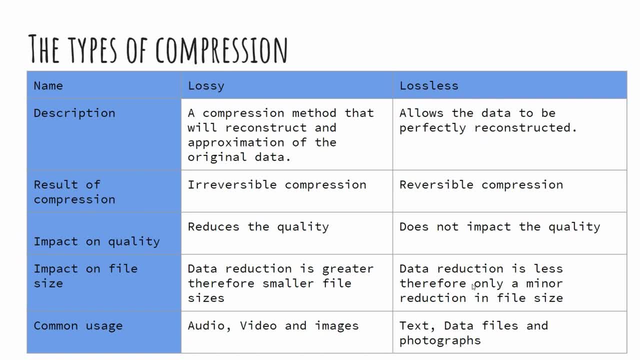 quite often you're still able to make out what's going on in that video and understand it without much challenge or complication. Now, when we start to look at other file types, this isn't the case, But generally speaking, audio and video and images are. 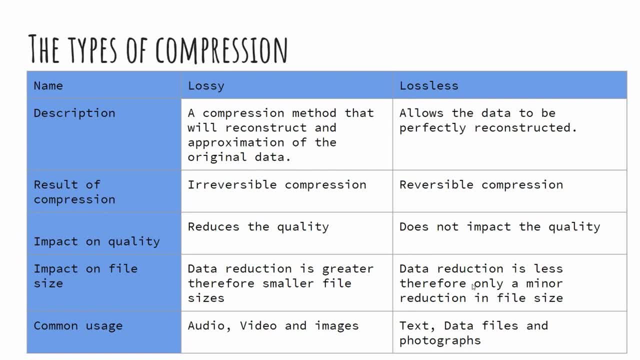 appropriate for this: lossy compression. You'll find, with lossy compression, whilst obviously you're losing data, you're also in a situation where it reduces the file size by a much greater amount as well. If we look at lossless compression, so the other type of compression, 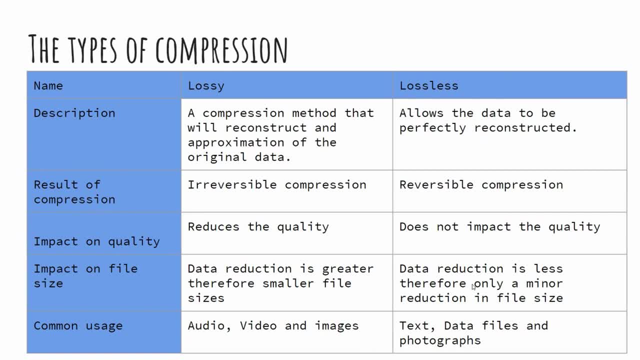 lossless. so you can remember this: by loses less. this is where the data is compressed, but you might find that you're able to actually reconstruct the entire file. So in that respect, when you compress, it's considered to be a reversible type of compression because it can. 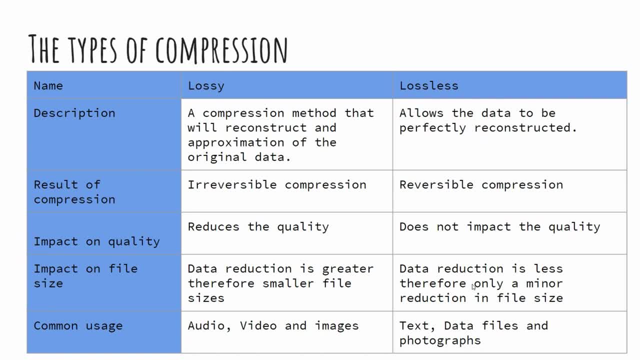 get straight back to the original quality of the file, So it doesn't impact quality when it's restored, But in doing so you lose a lot less data and therefore the file size isn't reduced as much, And this is a problem that we're going to talk about in a little bit. So if you're 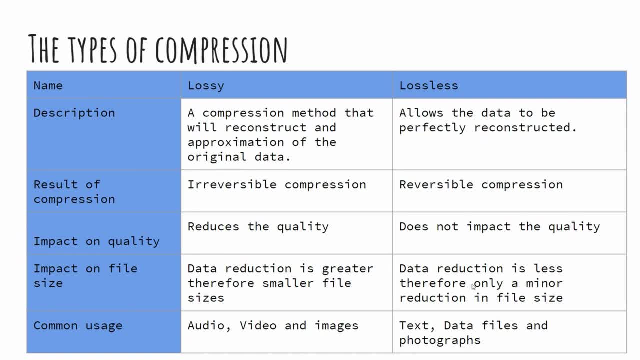 looking at lossy compression, it's appropriate for things like text and data files and high quality photographs, where you can't afford to lose information. So where in lossy compression, as we mentioned, you're actually deleting and removing data permanently, that's not. 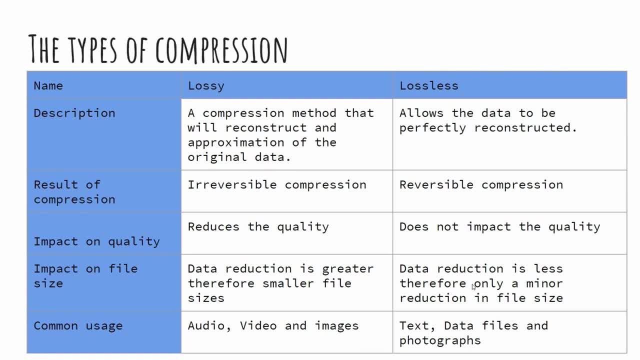 really appropriate for things like text files. you couldn't reduce the file size by reducing all of the vowels, so A, E, I, O and U, because it may not make the file at the end make any sense. So it is a case that you need to be mindful of the fact that these types of files 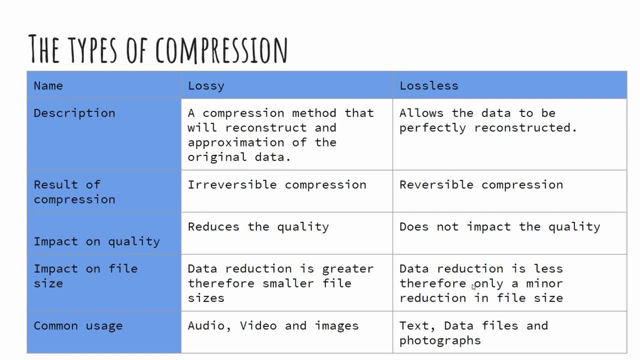 may need to be able to be restored back to their original file. So if you think about, for example, coding, if you were to compress your code and delete pieces of the code to reduce the file size, the code wouldn't then, in theory, run. So there are scenarios where 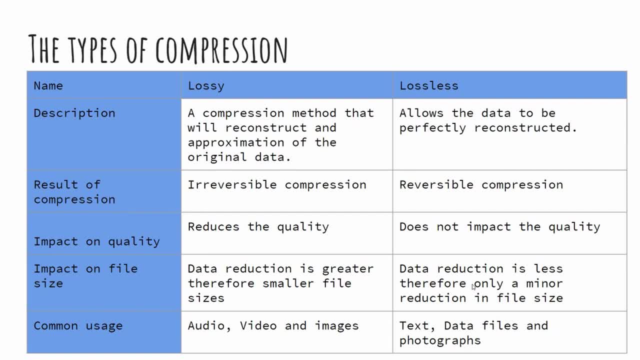 lossy and lossless are more appropriate, And it's, generally speaking, a kind of rule of thumb- is that if it's audio video or image, you can afford to lose some information with things like text or data files, And if you want a high quality photograph, then really.